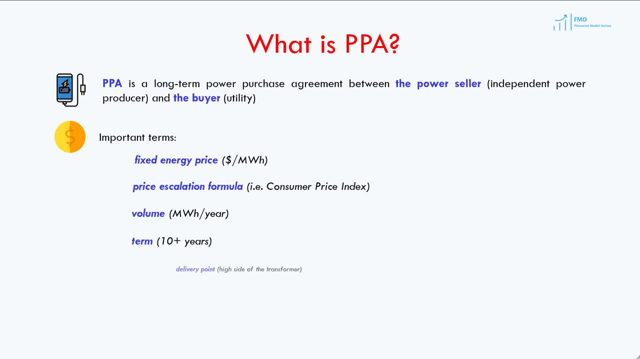 what will be the length of the contract and delivery point? where shall energy be delivered? The energy sales under the wind PPA and solar PPA are slightly different. Under the wind PPA, the off-taker has to purchase all of the energy. 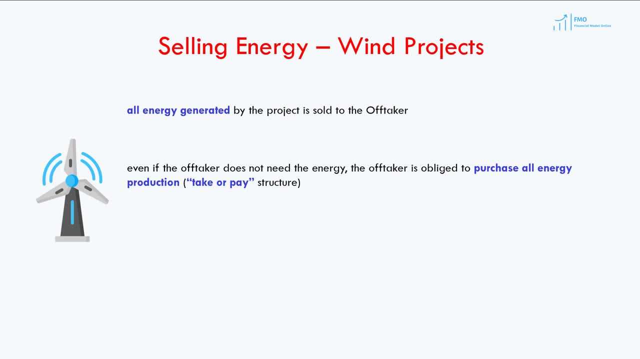 projects under the wind PPA, The off-taker has to purchase all of the energy projects under the produced by the wind project. Even if the off-taker does not need the energy, it has to pay the energy seller for the full amount of the energy produced. Therefore, the PPA for wind. 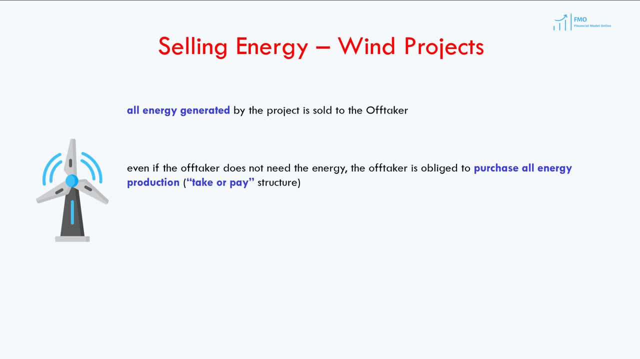 projects follow a take or pay structure. The off-taker has to take the delivery of the energy produced and pay, or even if it does not take the delivery, it still has to pay. Note that the off-taker requires the wind farm to maintain a certain percentage of mechanical availability. 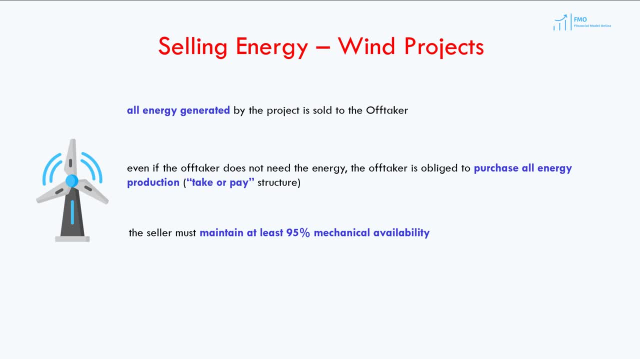 of the turbine, which is typically 95%. Failure to maintain required turbine availability results in liquidated damages, which are cash penalties payable to the off-taker. The PPA will include the formulas of how these liquidated damages need to be calculated If the failure 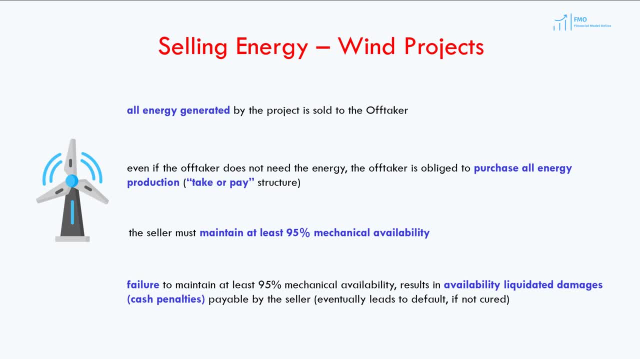 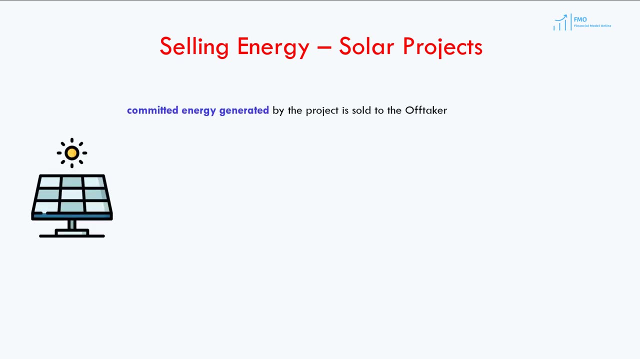 to maintain required turbine availability is not cured within a specified period, an event of default takes place under the PPA and the off-taker can terminate the PPA. The off-taker can terminate the PPA. Under the solar PPA, the off-taker must purchase the committed energy output, The committed energy. 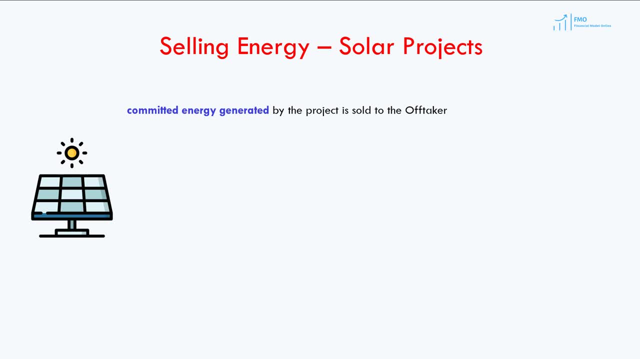 output is a forecasted energy output that will be sold to the off-taker. Similar to the wind PPA, solar PPA follows a take or pay structure. The off-taker is obliged to purchase committed energy production, even if the off-taker does not need the energy. Typically, the energy seller has 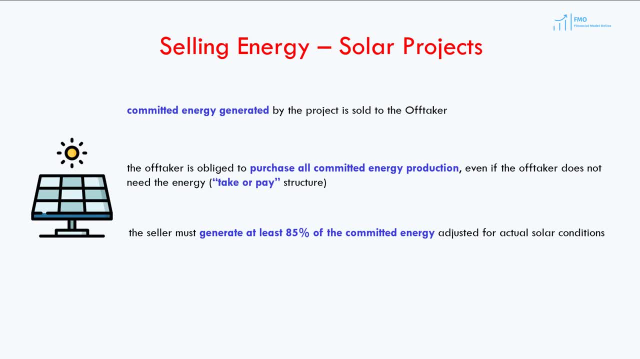 to be able to generate at least 85% of the committed energy output subject to the off-taker. The off-taker must be able to generate at least 85% of the committed energy output, subject to the solar conditions at the site. Failure to generate 85% of committed energy results in cash penalties. 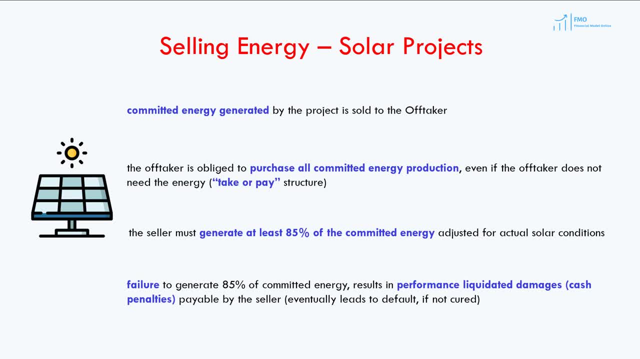 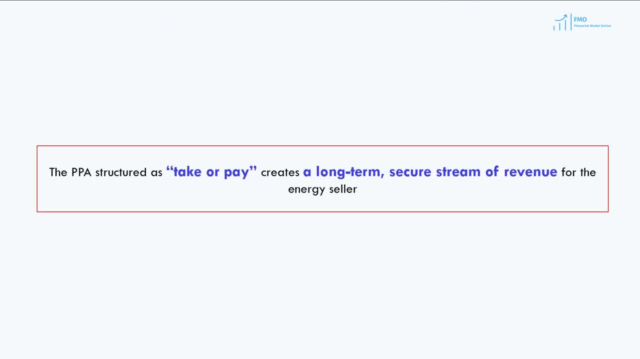 payable to the off-taker and, if not cured within a specified period, leads to a material breach of the PPA. So the PPA structured as take or pay contract creates a long-term secure stream of revenue for the energy seller, as long as the energy seller is able to fulfill. 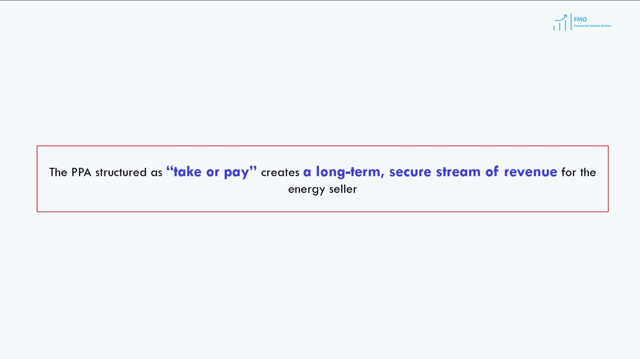 its obligation to maintain guaranteed availability In the case of the wind project, or generate committed energy output in case of the solar project. the energy sales is calculated following a simple formula: Energy price times actual energy output times. generation curtailment is equal to revenue. Note that for solar projects, 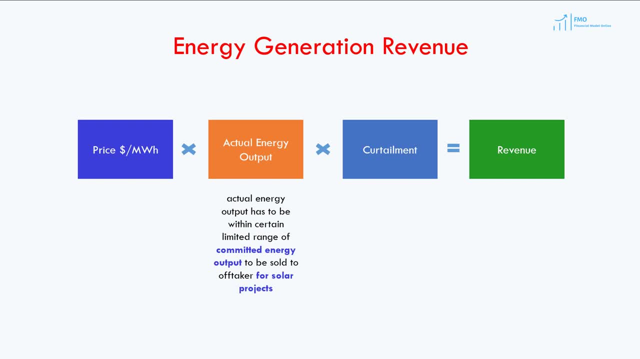 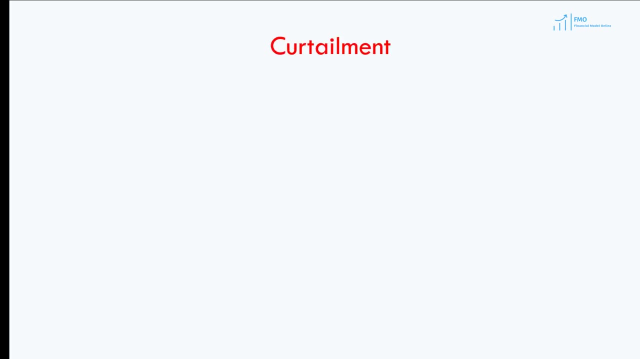 the actual energy output has to be within a certain limited range of committed energy output that we mentioned earlier. A curtailment is a reduction in the energy output on an involuntary basis and it can be compensable or non-compensable. Now let's take a look at curtailment. Non-compensable curtailment happens due to: 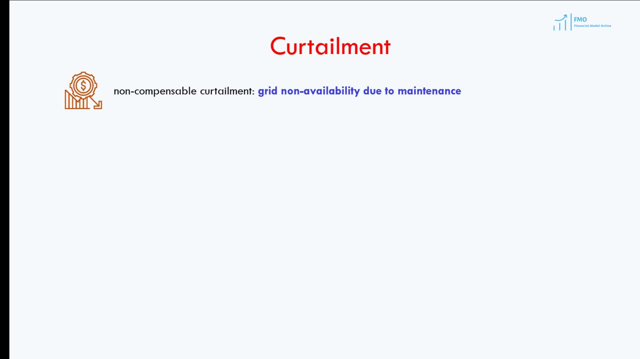 events outside the control of both the off-taker and energy seller. A typical example would be power transmission grid availability due to maintenance. when the grid cannot transmit the energy to the off-taker, A compensable curtailment happens because of the off-taker. 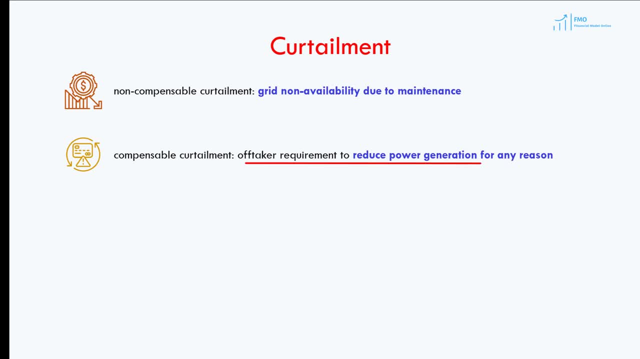 It is a situation when the off-taker cannot take the power from the energy seller for whatever reason other than non-compensable curtailment. The PPA will include a provision which describes the off-taker's right to require the energy seller to stop energy. 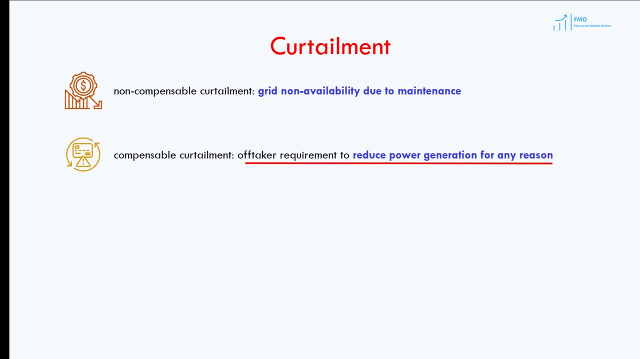 generation. An energy seller has to comply with such a requirement. The energy that could have been produced under a compensable curtailment is called deemed energy generation in the PPA, and the off-taker has to pay for deemed energy generation as if the energy has been delivered. 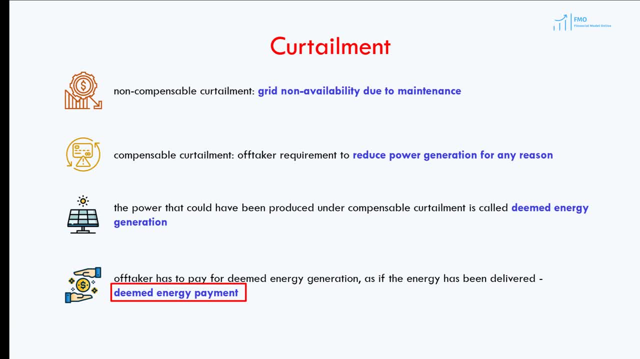 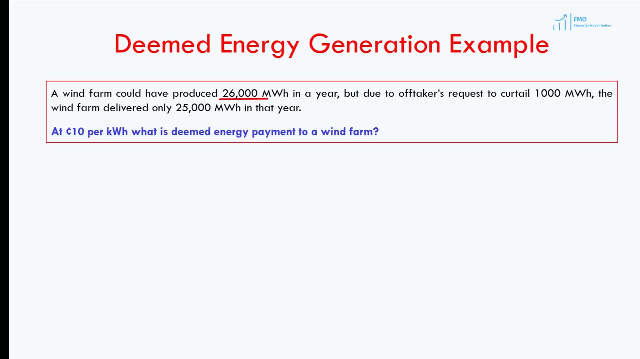 and such a payment is called off-taker. The off-taker has to pay for deemed energy generation, deemed energy payment. Let's review an example of deemed energy generation and payment. Suppose that a wind farm could have produced 26,000 MWh in a year, but due to offtakers' 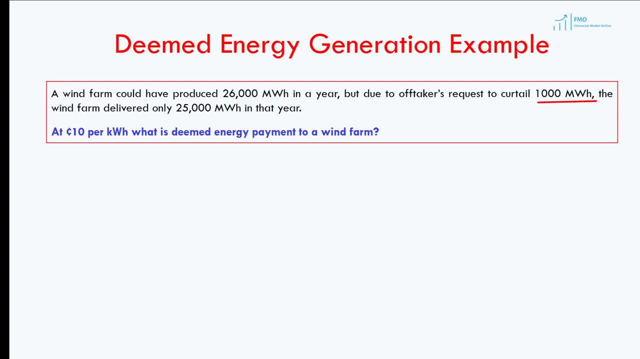 request to curtail 1,000 MWh. the wind farm delivered only 25,000 MWh in that year. The question is: at $0.10 per kWh, what is deemed energy payment to a wind farm? So the actual generation was 25,000 MWh. the energy price is $0.10 per kWh, which is $100 per 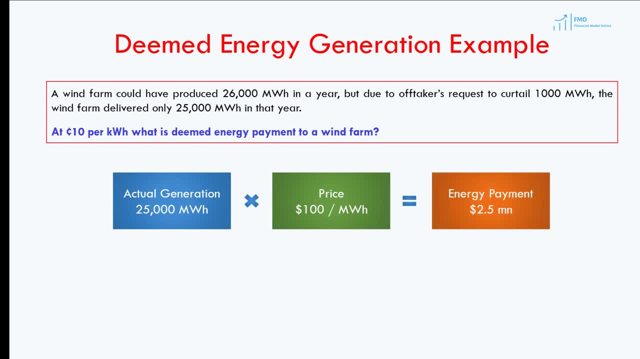 MWh and hence energy payment is 25,000 times 100, which is 2.5 million. The 1,000 MWh were curtailed as per the request from the offtaker and therefore the deemed energy generation is. 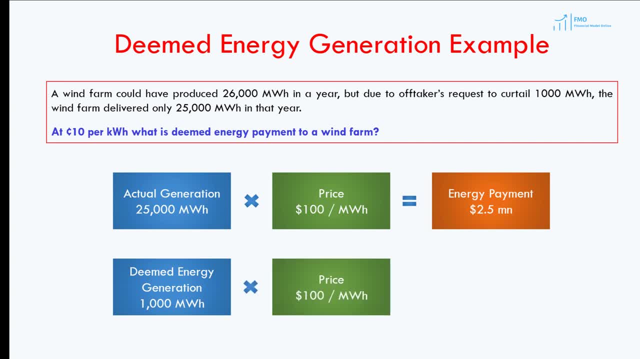 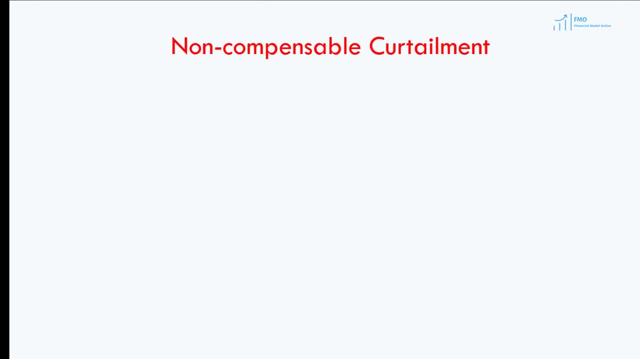 1,000.. The energy price is again 100, and 1,000 times 100 will get you $1,000.. So the offtaker has to compensate the energy seller for the curtailment. But how do we deal with non-compensable curtailment? 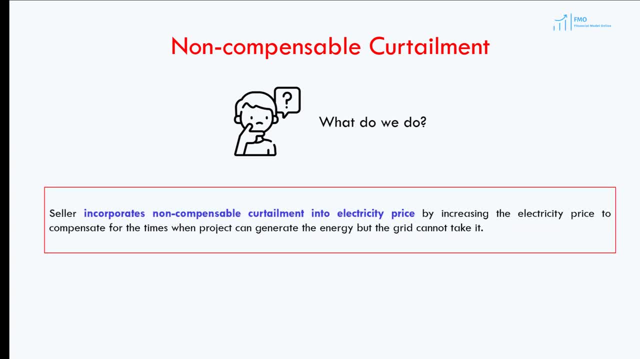 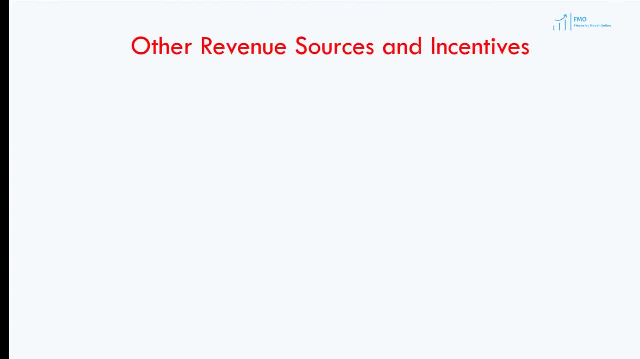 Usually, energy seller increases the energy price in the PPA to offset the estimated energy sales reduction because of the non-compensable curtailment, The PPA for renewables may also include additional revenue sources or in the futurerelated to the PPA for renewables. 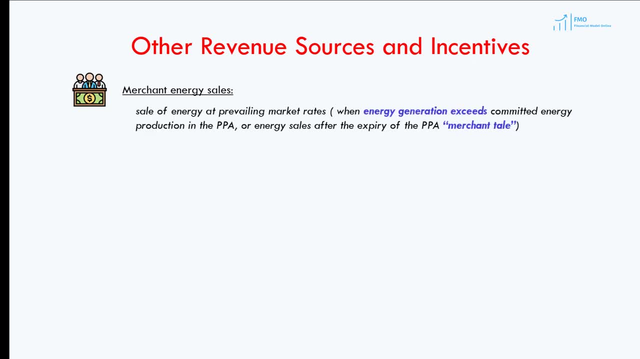 The PPA for renewables may also include additional revenue sources or, in the future, incentives. First, the power project may be producing energy above the committed energy production and this excess energy can be sold at market prevailing rates to the buyers other than the offtaker. 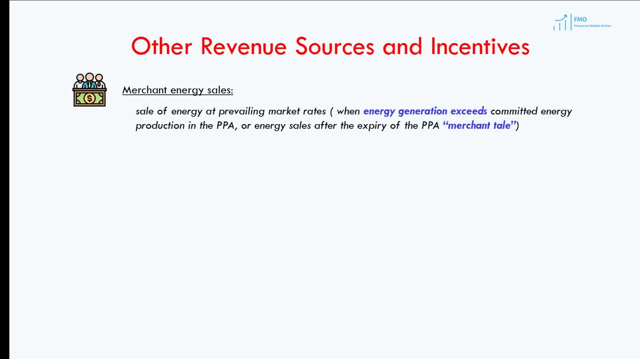 This is known as merchant energy sales. Second, the PPA term may be shorter than the life of the project, and energy generated in the periods after the PPA will also be sold at market prices to the buyers other than the offtaker. 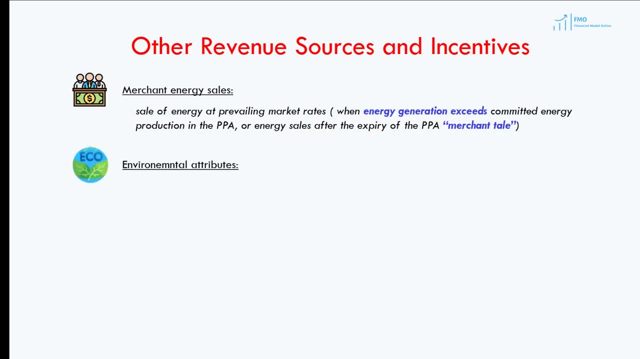 The period is called a merchant tail. PPA may include environmental attributes such as carbon credits. Typically, the offtaker also receives the carbon credits associated with the energy purchased from a renewable project. However, sometimes the PPA does not include sale and purchase of carbon credits and in 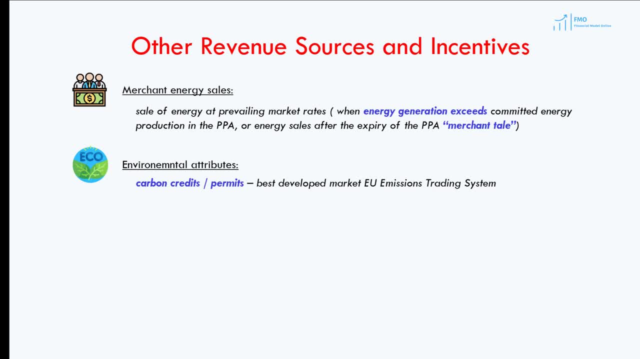 such a case, those carbon credits can be sold separately. Governments around the world have created subsidies and incentives for renewable projects. The prominent example would be investment, Investment tax credit and production tax credits in the USA, which have contributed significantly to renewable power development in the US power sector. 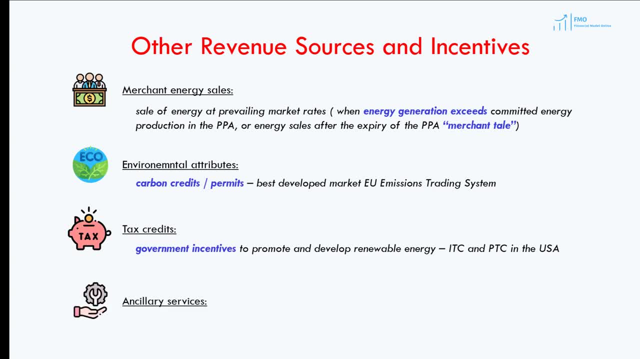 And finally, power projects may provide ancillary services, such as providing flexible generation to meet power outages or changing energy output to reflect short-term variations in supply and demand. The market has developed to procure and price these ancillary services in Europe and the 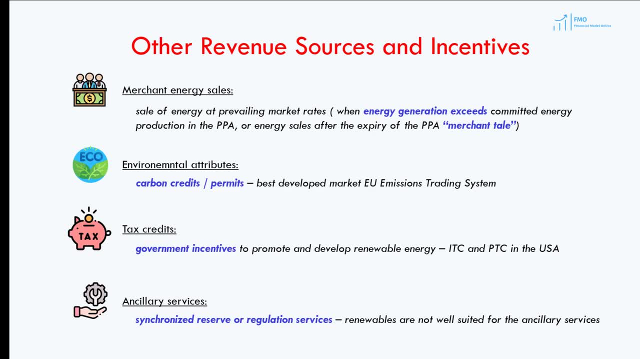 US. However, renewable energy projects are not well-suited to provide these services.